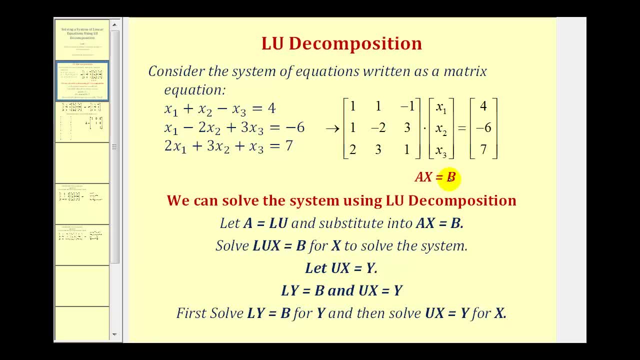 We can abbreviate this as a times x equals b. Now we can solve this system using LU decomposition, if we let the coefficient matrix, or matrix A, equal matrix L times matrix U, where L is a lower triangular matrix and U is an upper triangular matrix. 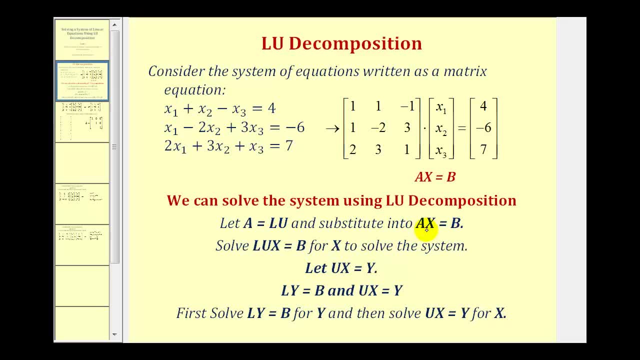 Then we can perform a substitution in the equation ax equals b. So if we substitute LU for A, we would have the equation L times U times x equals b, Which we can solve for x. if we let U times x equal y, We would solve the equation L times y equals b for y. 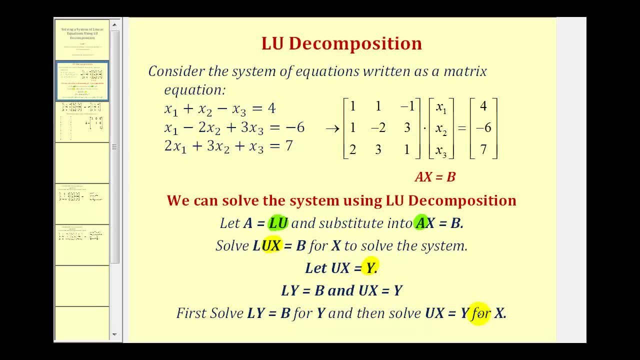 And then solve the equation: U times x equals y for x, which will give us our final solution. But the first step is to find the LU decomposition of the coefficient matrix. So, as an example, we're going to go ahead and solve this system here using LU decomposition. 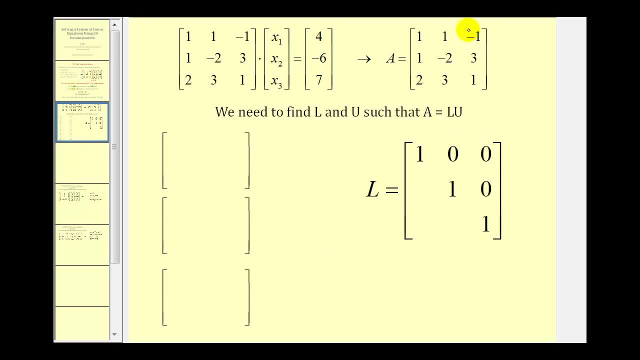 So again, here's our matrix equation and here's our coefficient matrix, which we want to find the LU decomposition for, And we'll do this using the shortcut method, where we'll perform row operations on this matrix to form the upper triangular matrix. 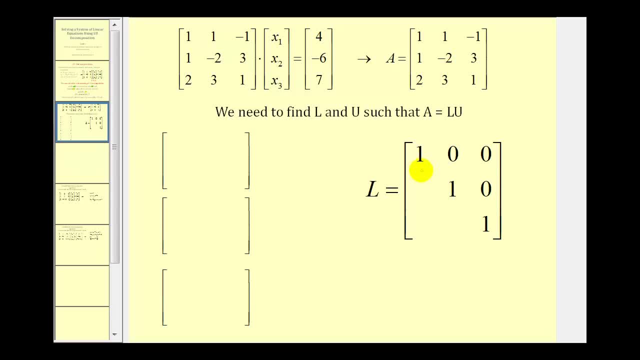 And at the same time, by using the opposite of the multipliers, we'll build the lower triangular matrix. So, for example, if we want to have a zero in this position here, we want to determine what multiple of another row we would add to this row to have this element be a zero. 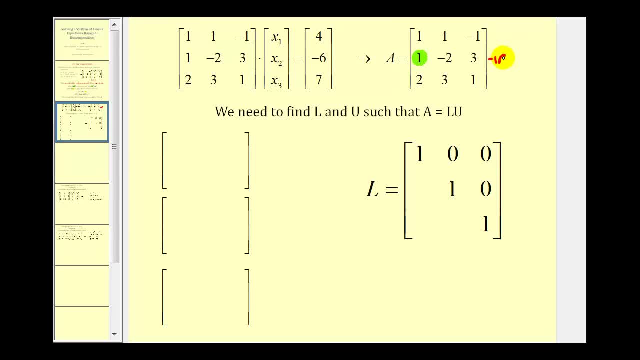 So we're going to replace row two with negative one times row one plus row two. Let's go ahead and do that and place our new matrix over here on the left, So row one and row three will stay the same, And then for row two, negative one times one plus one is zero. 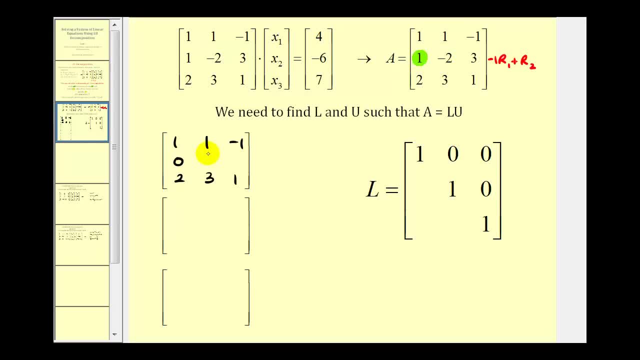 Negative one times one plus negative two is negative three. Negative one times negative one plus three is positive four. Now we use the multiplier of negative one to help us obtain a zero in row two, column one, Which means the element in row two, column one of our lower triangular matrix. 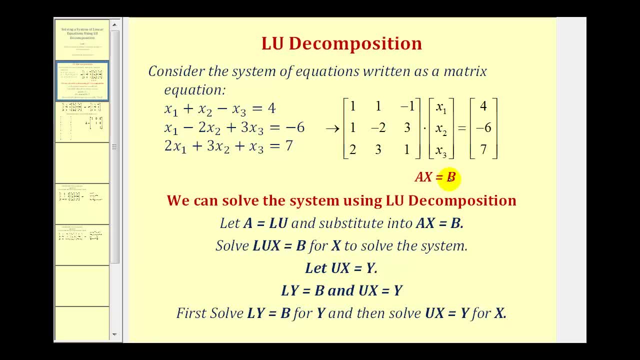 We can abbreviate this as a times x equals b. Now we can solve this system using LU decomposition, if we let the coefficient matrix, or matrix A, equal matrix L times matrix U, where L is a lower triangular matrix and U is an upper triangular matrix. 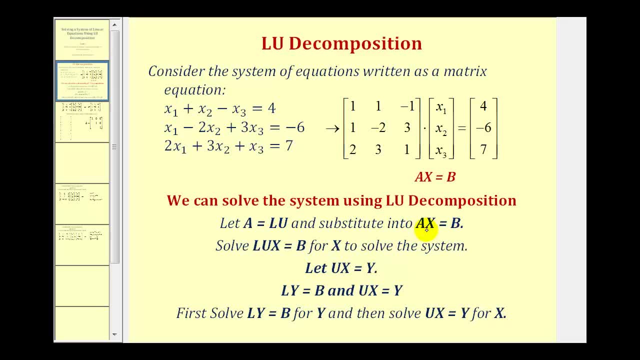 Then we can perform a substitution in the equation ax equals b. So if we substitute LU for A, we would have the equation L times U times x equals b, Which we can solve for x. if we let U times x equal y, We would solve the equation L times y equals b for y. 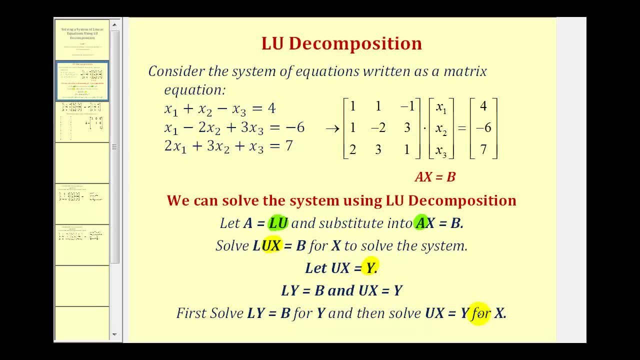 And then solve the equation: U times x equals y for x, which will give us our final solution. But the first step is to find the LU decomposition of the coefficient matrix. So, as an example, we're going to go ahead and solve this system here using LU decomposition. 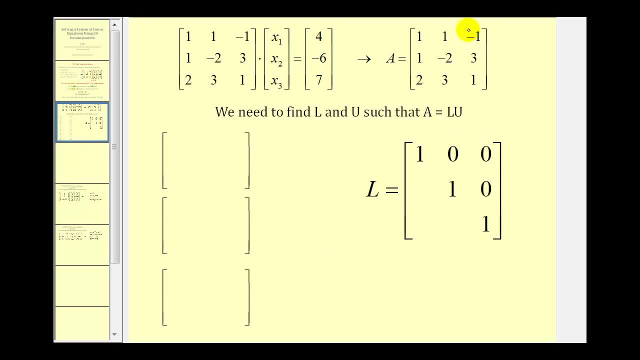 So again, here's our matrix equation and here's our coefficient matrix, which we want to find the LU decomposition for, And we'll do this using the shortcut method, where we'll perform row operations on this matrix to form the upper triangular matrix. 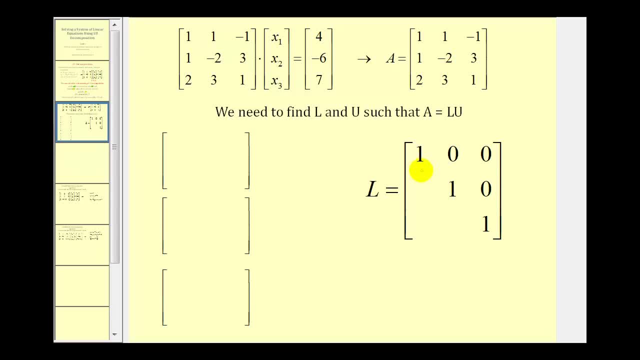 And at the same time, by using the opposite of the multipliers, we'll build the lower triangular matrix. So, for example, if we want to have a zero in this position here, we want to determine what multiple of another row we would add to this row to have this element be a zero. 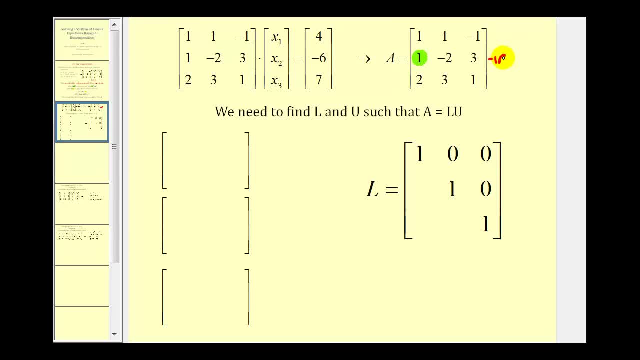 So we're going to replace row two with negative one times row one plus row two. Let's go ahead and do that and place our new matrix over here on the left, So row one and row three will stay the same, And then for row two, negative one times one plus one is zero. 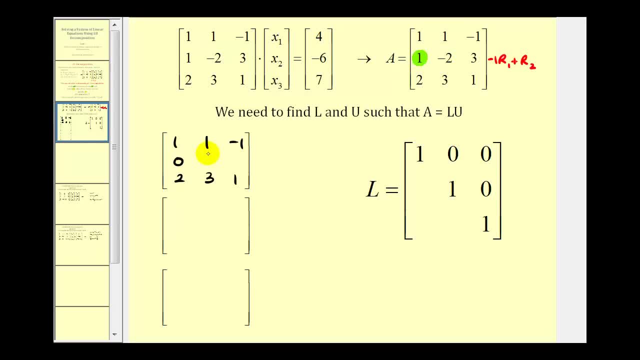 Negative one times one plus negative two is negative three. Negative one times negative one plus three is positive four. Now we use the multiplier of negative one to help us obtain a zero in row two, column one, Which means the element in row two, column one of our lower triangular matrix. 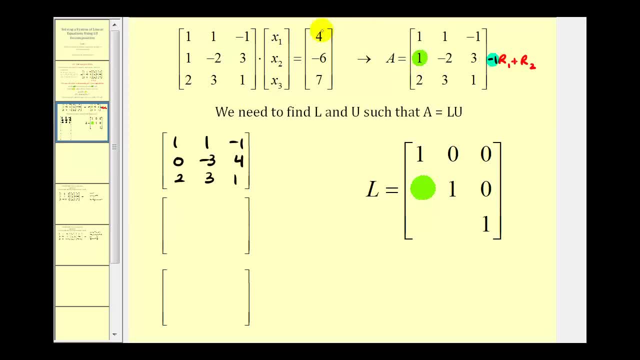 will be the opposite of our multiplier, or the opposite of negative one. So this element here will be positive one. Now let's obtain a zero in this position here, or row three, column one. We can replace row three with negative, two times row one plus row three. 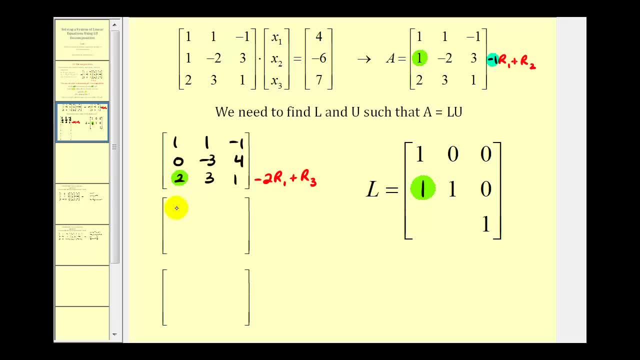 to obtain a zero here Again, notice- the first two rows would stay the same. So we have negative two times one plus two is zero. Negative two times one plus three is positive one And negative two times negative. one is positive. two plus one is positive three. 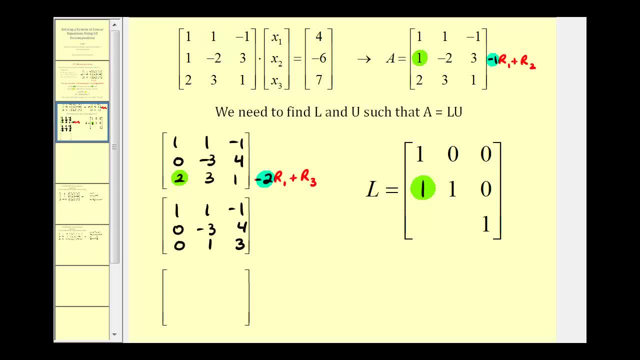 Our multiplier is negative two, To obtain a zero in row three, column one, Which means row three, column one of our lower triangular matrix will be the opposite of negative two, Which means this will be positive two. And for the last row operation we want a zero here. 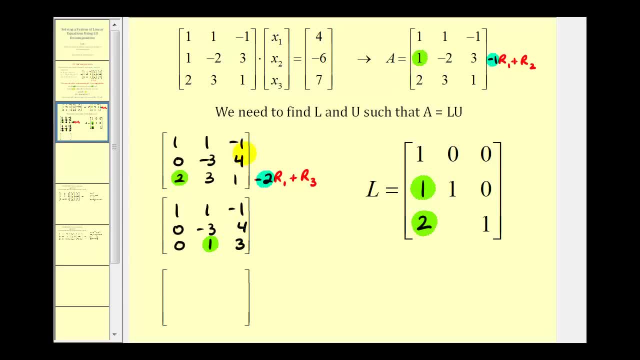 But we have to use row two to do that. So if we replace, so if we replace row three with one third times row two plus row three, this will give us a zero here. First two rows stay the same. This element will still be zero. 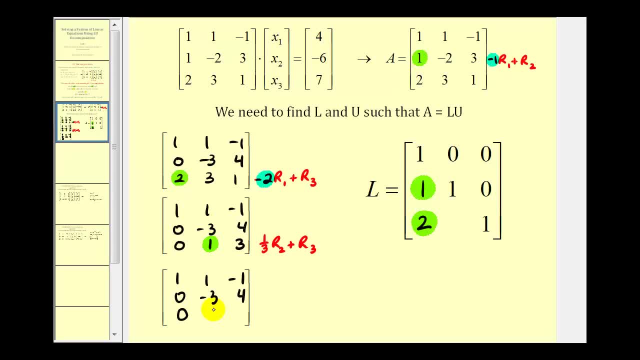 And then here we'll have one third times negative three, That's negative one, plus one that's zero. And for this last element we'll have one third times four, That's four thirds Plus positive three, which happens to be nine thirds. 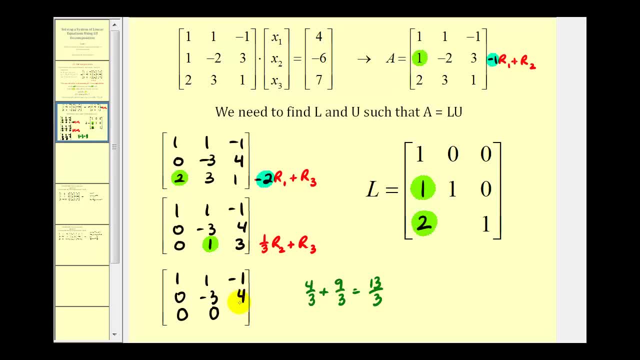 So the last element here will be thirteen thirds. Our multiplier to obtain a zero in row three, column two, Which corresponds to this position here in L, Is going to be the opposite of positive one third, Which means this element here will be negative one third. 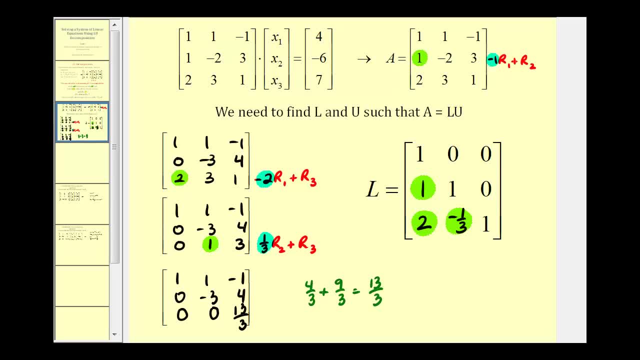 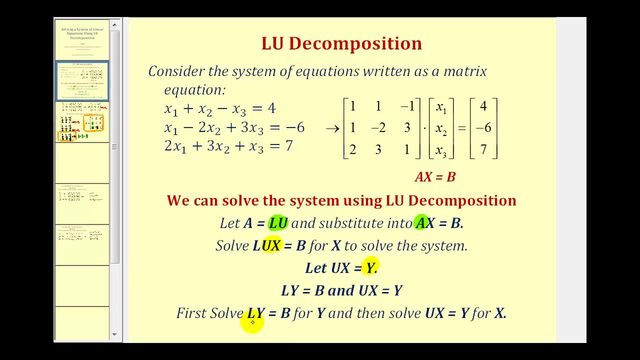 So now we have the LU decomposition of matrix A. Here's our upper triangular matrix And here's our lower triangular matrix. So now, if we go back to our notes just for a moment, We're going to solve the equation. L times Y equals B for Y. 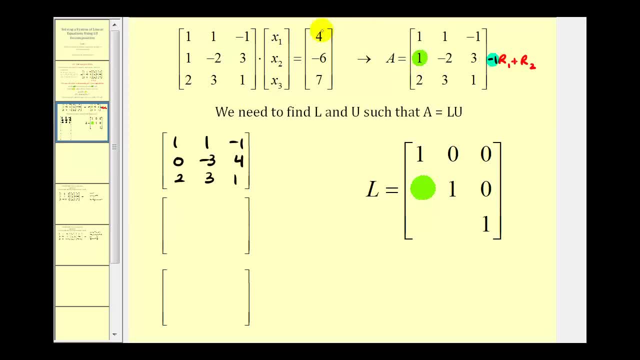 will be the opposite of our multiplier, or the opposite of negative one. So this element here will be positive one. Now let's obtain a zero in this position here, or row three, column one. We can replace row three with negative, two times row one plus row three. 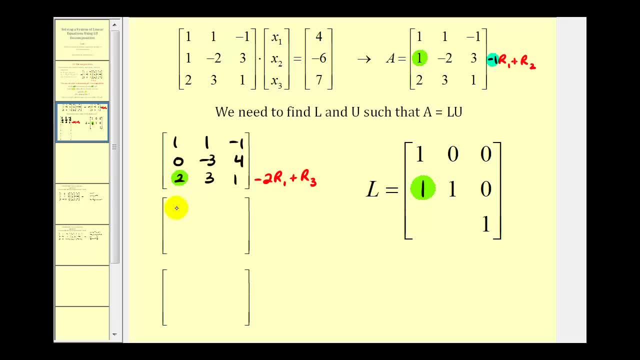 to obtain a zero here Again, notice- the first two rows would stay the same. So we have negative two times one plus two is zero. Negative two times one plus three is positive one And negative two times negative. one is positive. two plus one is positive three. 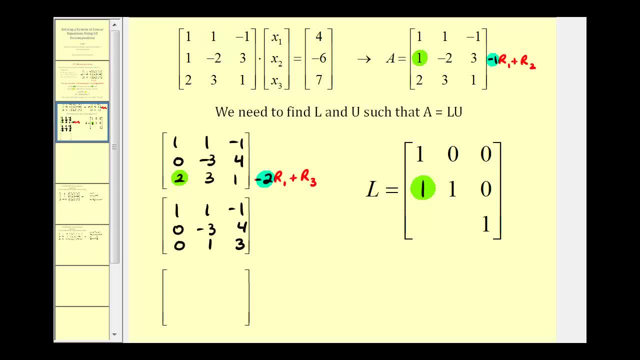 Our multiplier is negative two, To obtain a zero in row three, column one, Which means row three, column one of our lower triangular matrix will be the opposite of negative two, Which means this will be positive two. And for the last row operation we want a zero here. 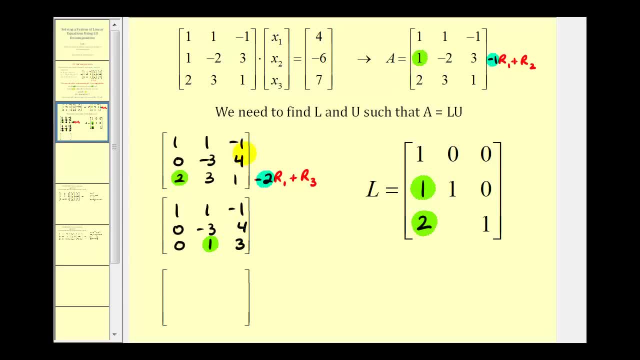 But we have to use row two to do that. So if we replace, so if we replace row three with one third times row two plus row three, this will give us a zero here. First two rows stay the same. This element will still be zero. 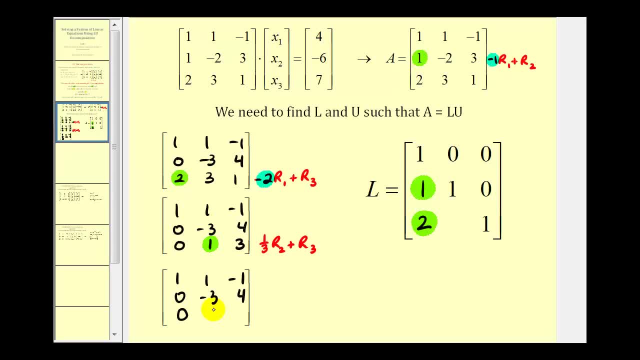 And then here we'll have one third times negative three, That's negative one, plus one that's zero. And for this last element we'll have one third times four, That's four thirds Plus positive three, which happens to be nine thirds. 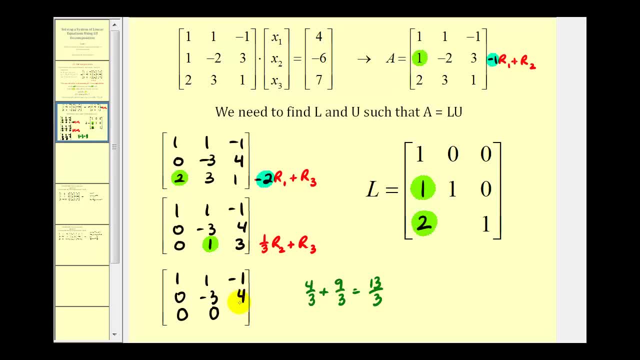 So the last element here will be thirteen thirds. Our multiplier to obtain a zero in row three, column two, Which corresponds to this position here in L, Is going to be the opposite of positive one third, Which means this element here will be negative one third. 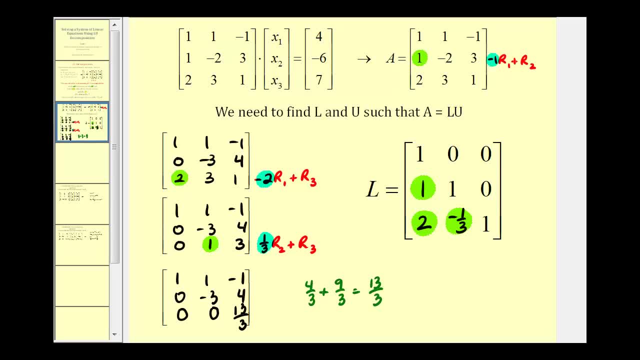 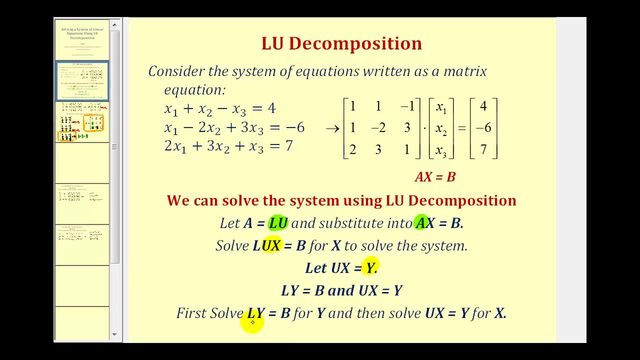 So now we have the LU decomposition of matrix A. Here's our upper triangular matrix And here's our lower triangular matrix. So now, if we go back to our notes just for a moment, We're going to solve the equation. L times Y equals B for Y. 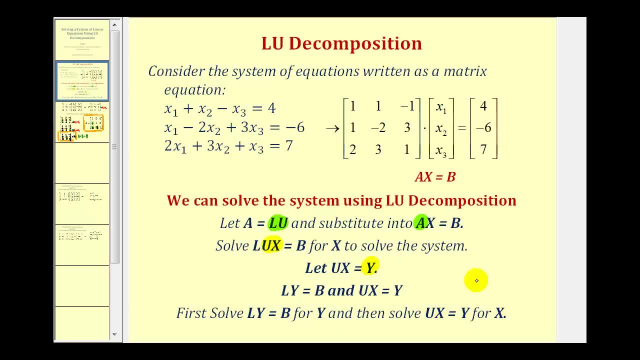 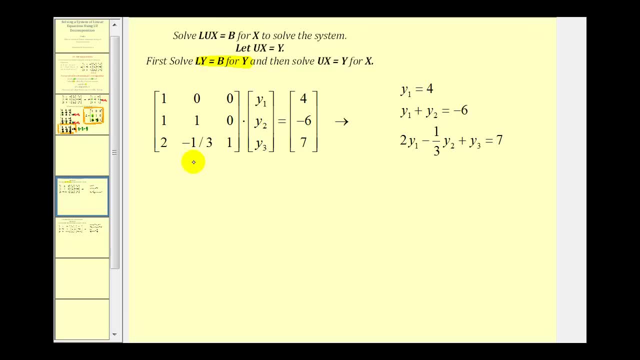 And then U times X equals Y for X. So here's our equation: L times Y equals B. Here's our lower triangular matrix, Which we built using the shortcut. Here's the matrix Y And here's our matrix B. So we write this back as equations: 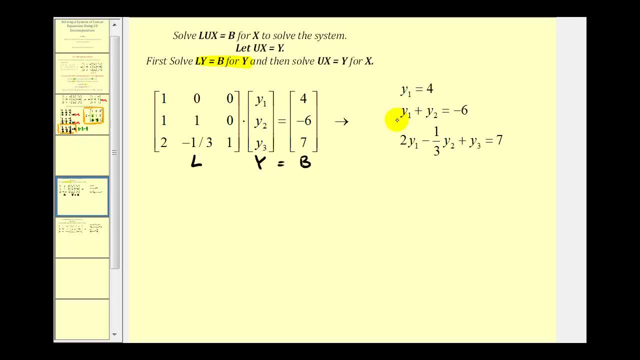 We would have: Y sub one equals four. Y sub one plus Y sub two equals negative six. Two times Y sub one minus one third. Y sub two plus Y sub three equals seven. So we can see: Y sub one is equal to four. 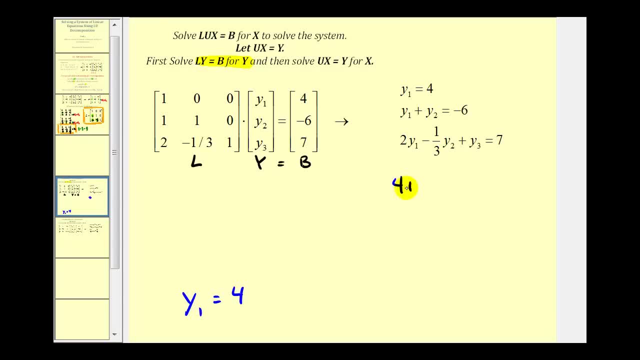 Well, if Y sub one is equal to four, We would have four plus Y sub two equals negative six. So Y sub two equals negative ten. And then for Y sub three- We have a little bit of work to do- We would have two times Y sub one, which is eight. 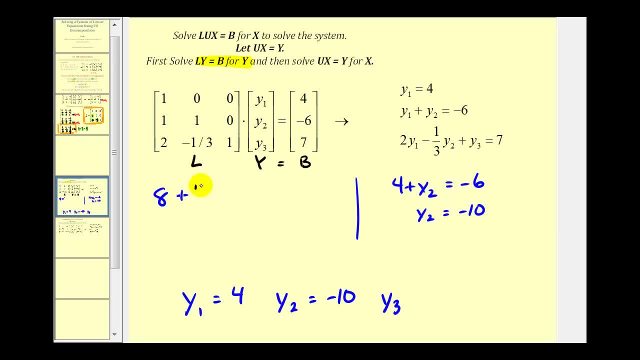 Minus one third times negative ten. That's plus ten thirds. Plus Y sub three Equals seven. So now we have Y sub three Equals seven minus eight. That's negative one Minus ten thirds. It's going to be negative thirteen thirds. 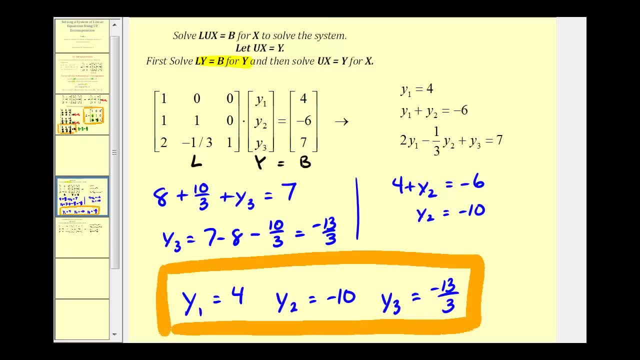 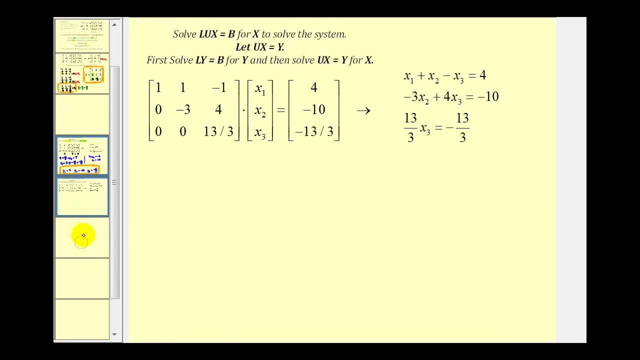 Now that we have the values of the elements in matrix Y, Our last step is to solve the equation: U times X equals Y for X. And here's that matrix equation. Notice: this is our upper triangular matrix which we found. Here's our matrix X. 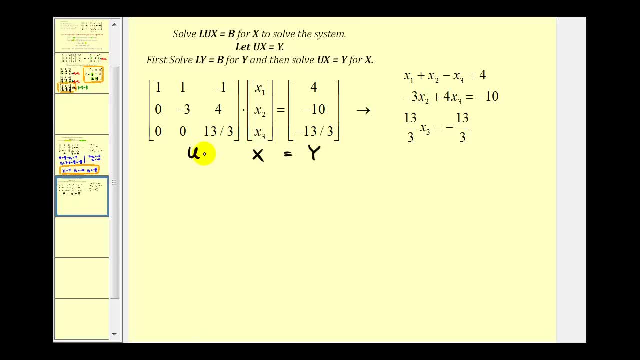 And here's our matrix Y with the values that we just found. So if we write this as equations, We would have: X sub one plus X sub two minus X sub three equals four Negative three. X sub two plus four. X sub three equals negative ten. 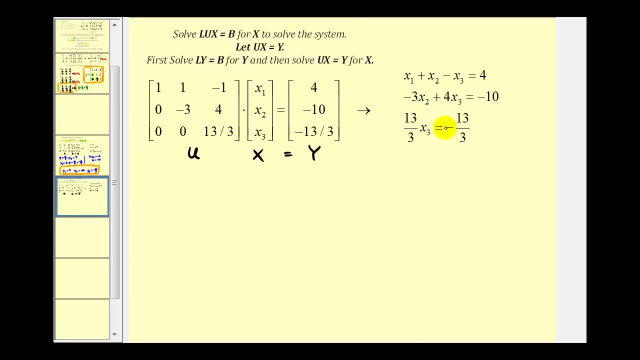 And the last equation is: Thirteen thirds. X sub three equals Negative thirteen thirds. So hopefully we can see that X sub three is equal to Negative one. So if X sub three is equal to negative one, The second equation would be: 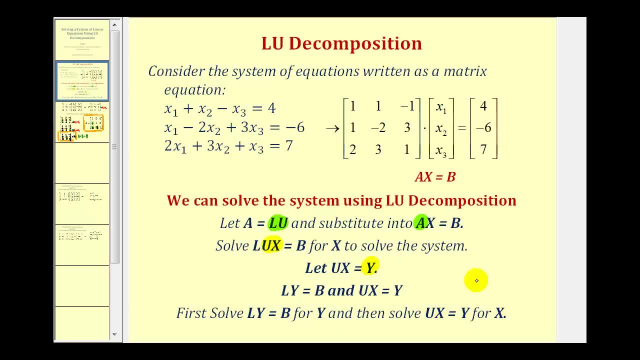 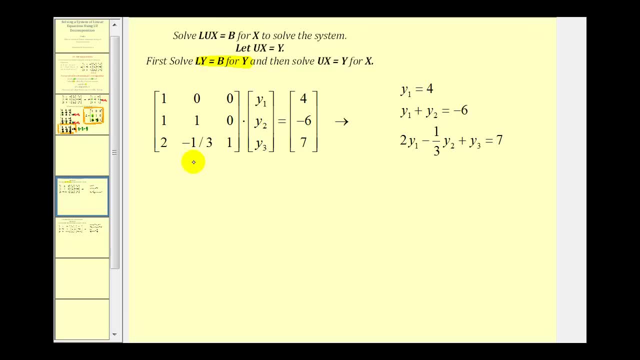 And then U times X equals Y for X. So here's our equation: L times Y equals B. Here's our lower triangular matrix, Which we built using the shortcut. Here's the matrix Y And here's our matrix B. So we write this back as equations: 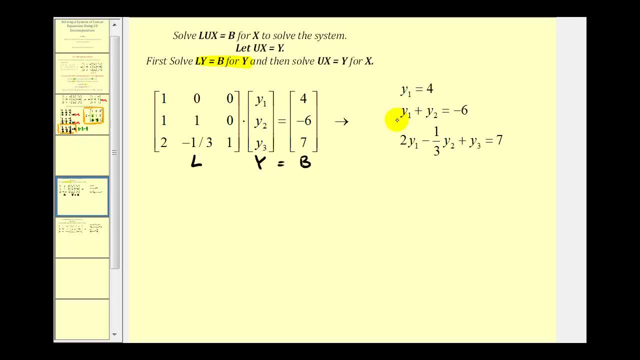 We would have: Y sub one equals four. Y sub one plus Y sub two equals negative six. Two times Y sub one minus one third. Y sub two plus Y sub three equals seven. So we can see: Y sub one is equal to four. 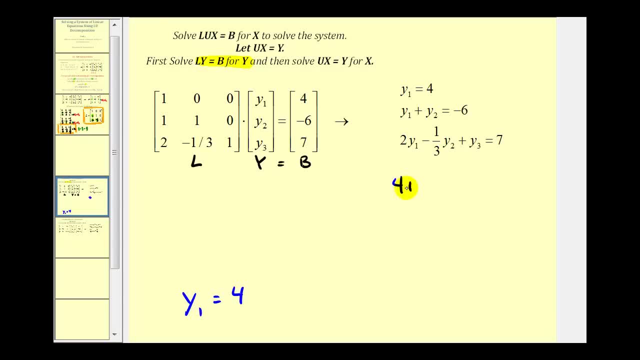 Well, if Y sub one is equal to four, We would have four plus Y sub two equals negative six. So Y sub two equals negative ten. And then for Y sub three- We have a little bit of work to do- We would have two times Y sub one, which is eight. 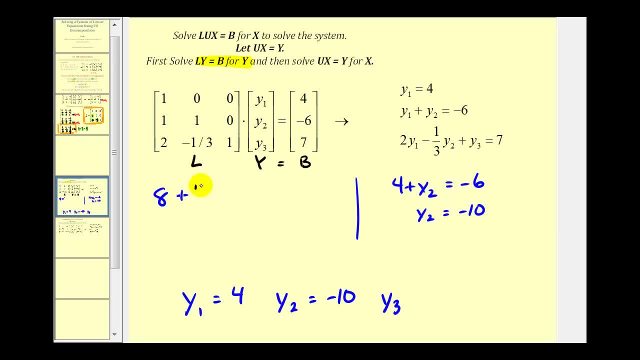 Minus one third times negative ten. That's plus ten thirds. Plus Y sub three Equals seven. So now we have Y sub three Equals seven minus eight. That's negative one Minus ten thirds. It's going to be negative thirteen thirds. 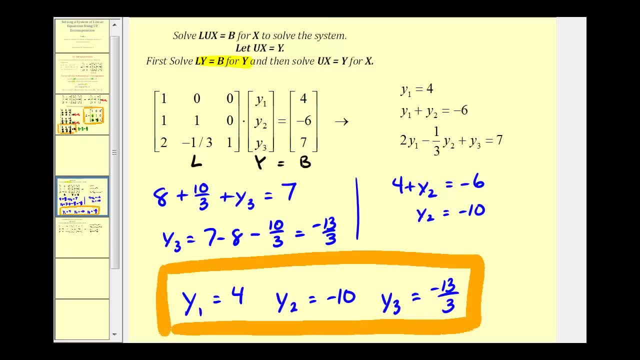 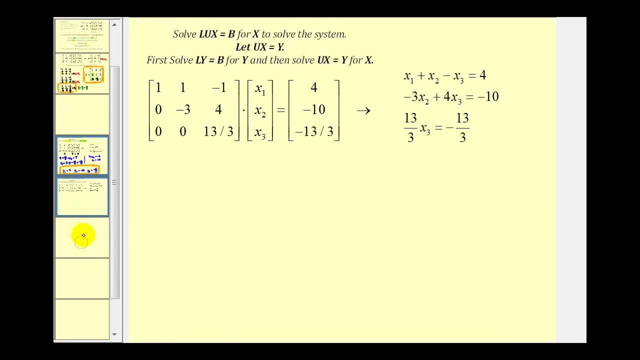 Now that we have the values of the elements in matrix Y, Our last step is to solve the equation: U times X equals Y for X. And here's that matrix equation. Notice: this is our upper triangular matrix which we found. Here's our matrix X. 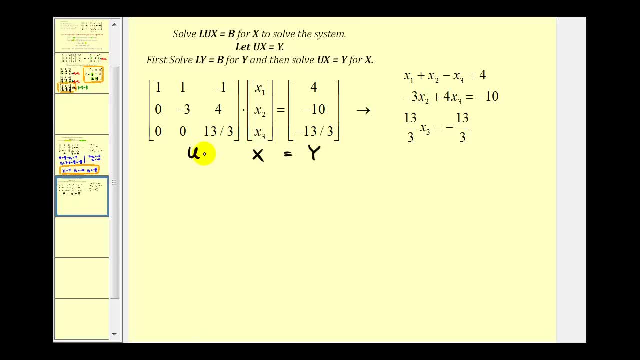 And here's our matrix Y with the values that we just found. So if we write this as equations, We would have: X sub one plus X sub two minus X sub three equals four Negative three. X sub two plus four. X sub three equals negative ten. 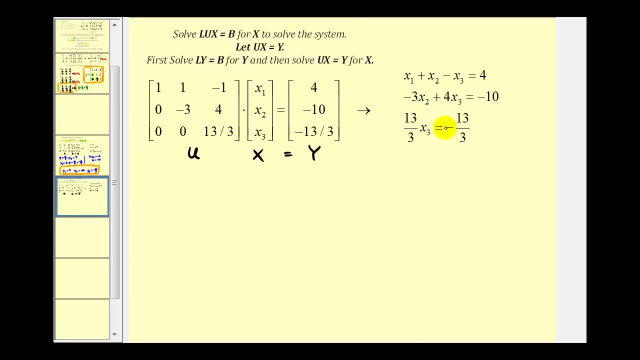 And the last equation is: Thirteen thirds. X sub three equals Negative thirteen thirds. So hopefully we can see that X sub three is equal to Negative one. So if X sub three is equal to negative one, The second equation would be: